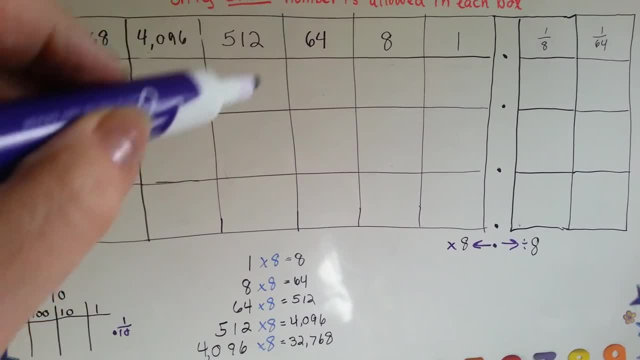 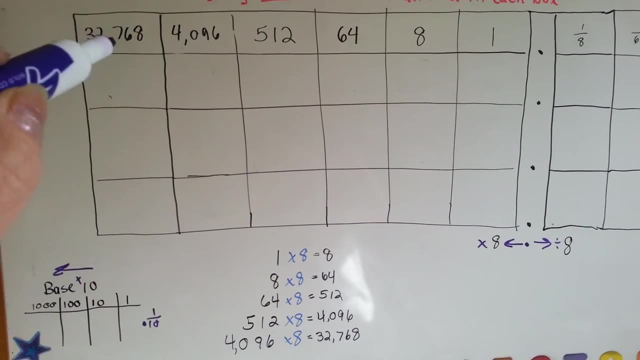 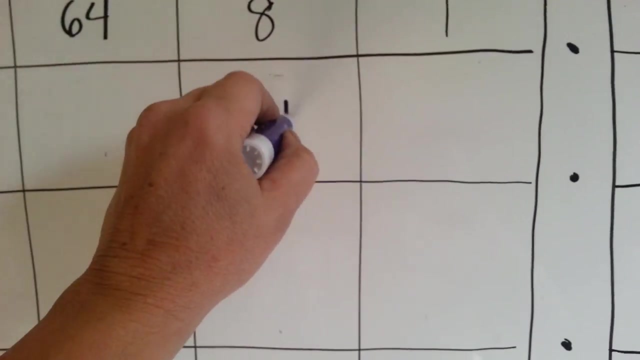 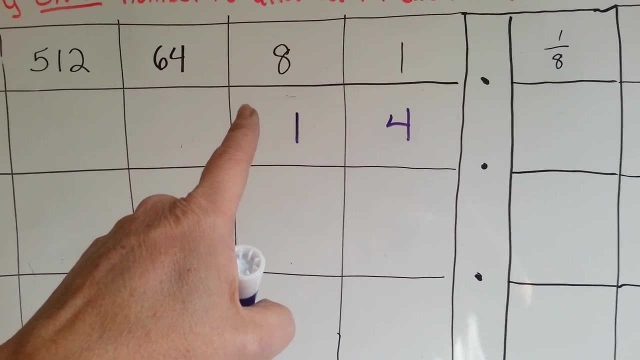 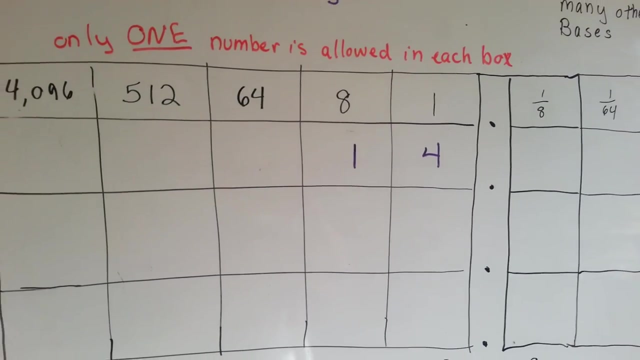 1 times 8 is 8.. 8 times 8 is 64.. 64 times 8 is 512.. 512 times 8 is 4096, and so on, And we would just keep going this way, Multiplying this number by 8.. So if I said that you've got this number in base 8, it means you have 1, 8 and 4 1s. 1, 8 and 4 1s would be 12 to our place value base 10 system. 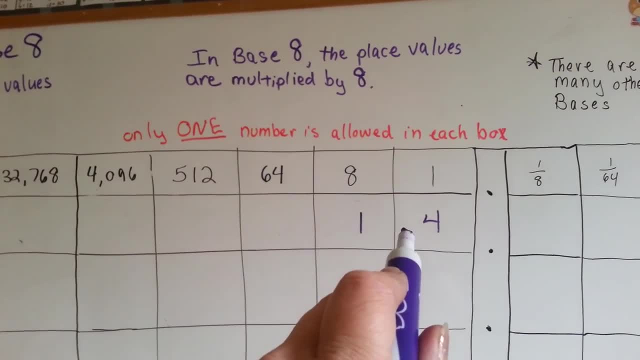 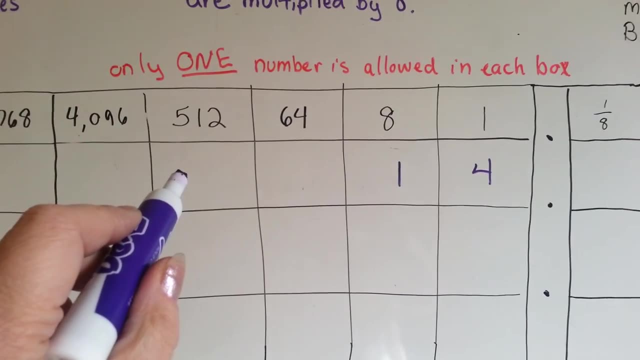 But in base 8, it would be written as a 1 and a 4.. Let's say you had the number 4 and a 4. 513.. What you would do is you would put a 1 here for 512. 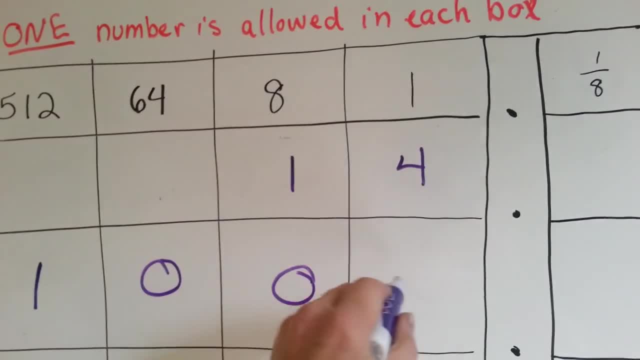 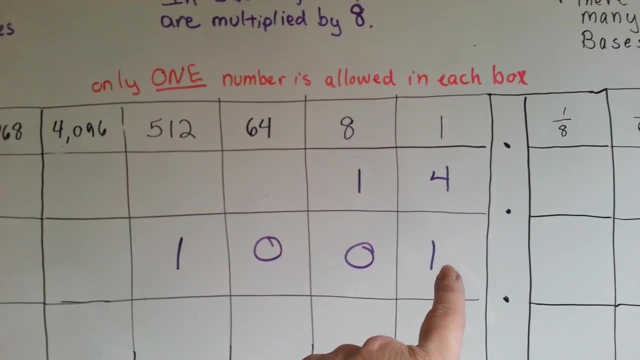 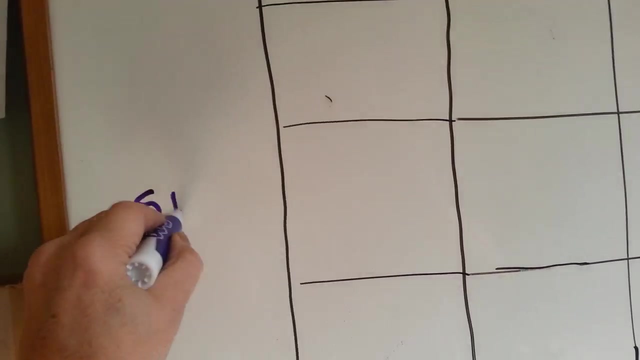 Okay, No 64s, no 8s, but a 1, because you've got 513.. You get 512 plus 1 more, So to say 513,, you say 1001.. 513 would equal 1001. 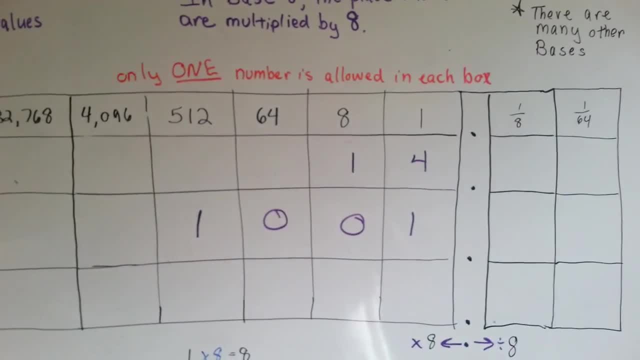 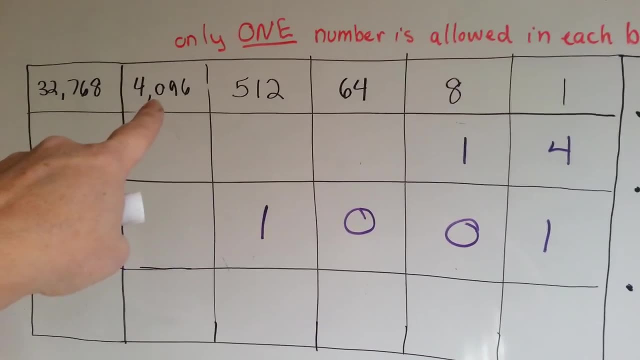 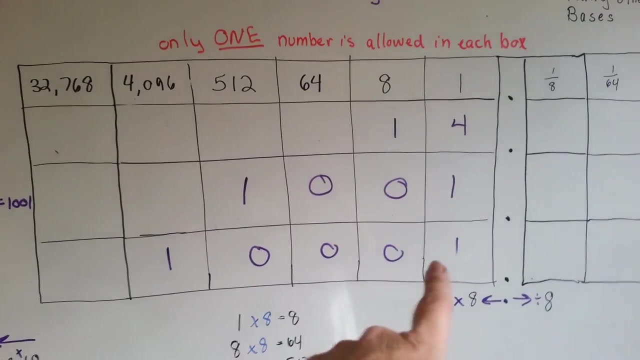 in base 8.. See how that works. If you had 497, you'd get 1 of these, 0 of these and a 1.. To get 4097.. See how that worked. So you multiply by 8 on this side of the decimal point. 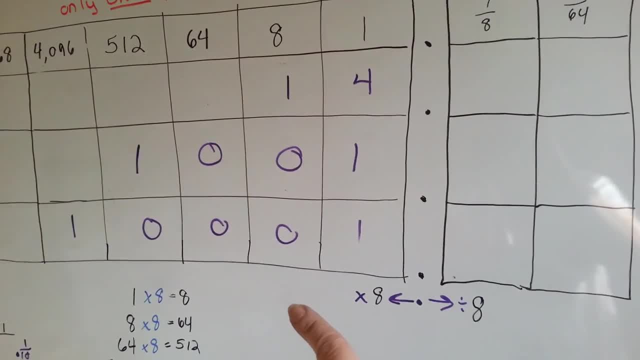 You divide by 8 on the right side of the decimal point. So these are the numbers. So you multiply by 8 on this side of the decimal point. You divide by 8 on the right side of the decimal point. So these are the numbers. 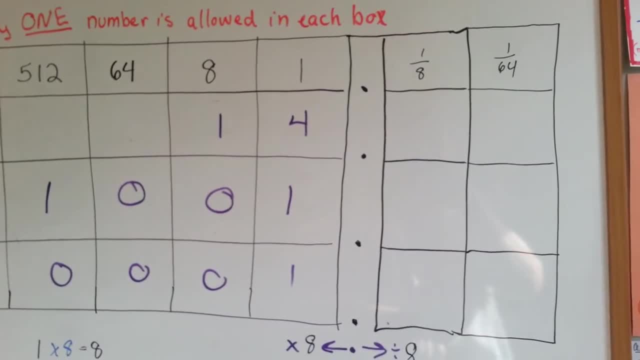 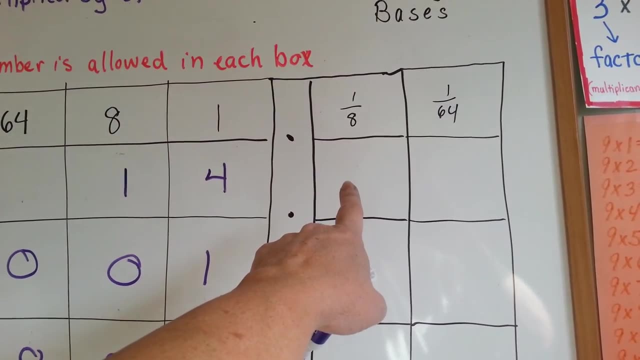 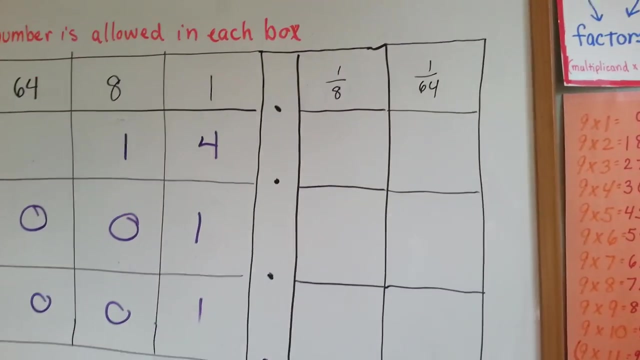 So these would be 8s. So if you had 3 8s, it would be in this column. Once you got smaller, it would get into 64ths. It would be in this column, And that's how the fractions and decimals would be set up. 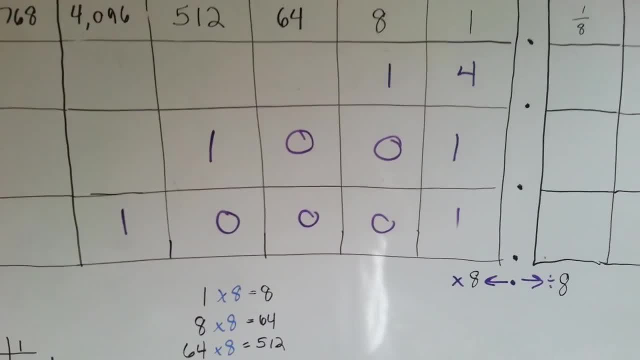 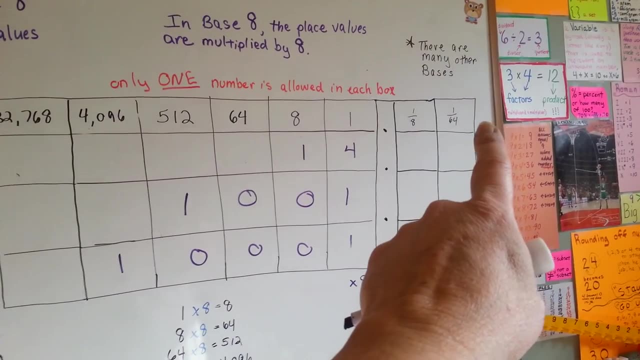 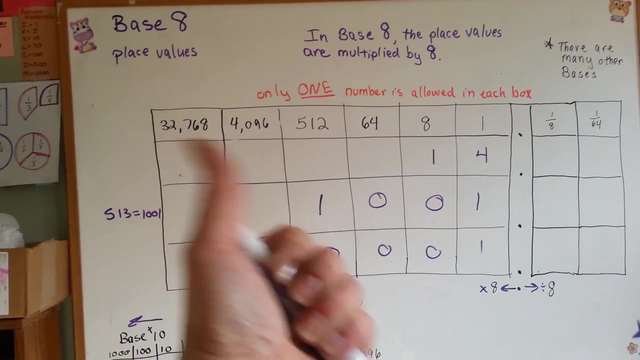 on the right side of the decimal point And it would get smaller and smaller. You'd go from 64ths to 512ths As the next column over. So that's base 8.. Just keep multiplying on the left of the decimal point.